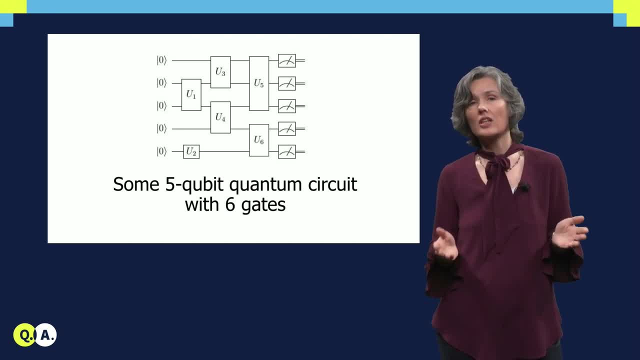 fixed, typically thermal, state. So how to make the failure probability per gate low, for example, as low as 10 to the minus 15?? For none of the qubits under current investigation like the ones that you'll hear about the. 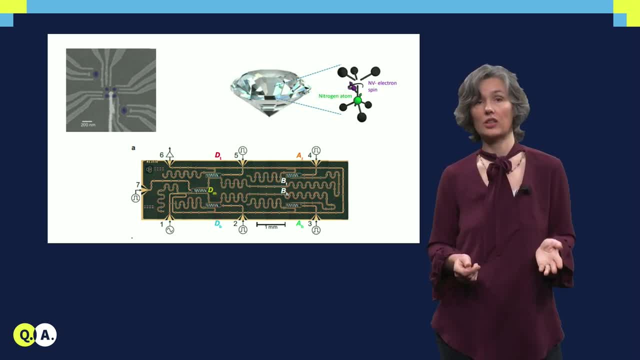 failure rate of a single or two qubit gate is less than, say, one percent. The past 20 years have seen a lot of progress in making better qubits with longer lifetimes and better gates. but to reach 10 to the minus 15 by hardware advances just seems implausible. 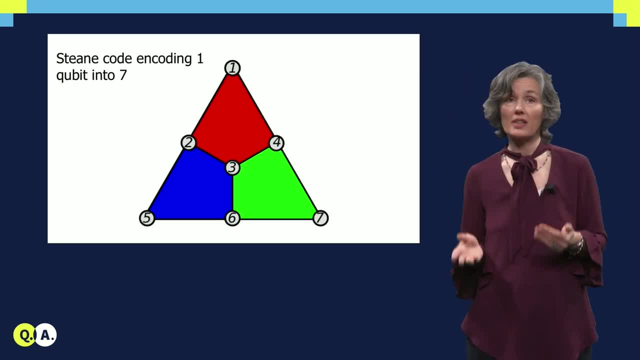 Now the idea of quantum error correction is to represent quantum error. We represent quantum information redundantly. For example, instead of a single qubit, we use seven qubits, And these seven qubits together constitute one new so-called logical qubit. 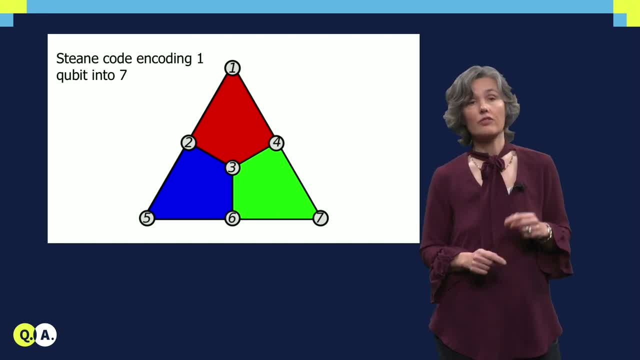 And on this logical qubit we operate as follows: First, we constantly monitor for errors on any of these seven qubits. We can't do this by measuring these qubits- Why not? Otherwise we lose their state. Instead, we'll actually include an error. 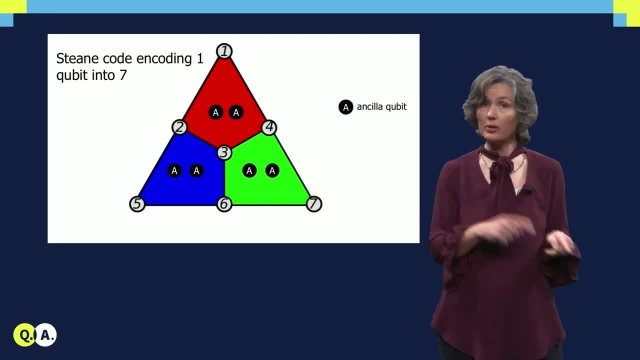 We include ancilla or helper qubits which we couple to the data qubit and we'll only read out the ancilla qubits And with this error information we infer what errors have happened. In this way we can undo or reverse these errors. 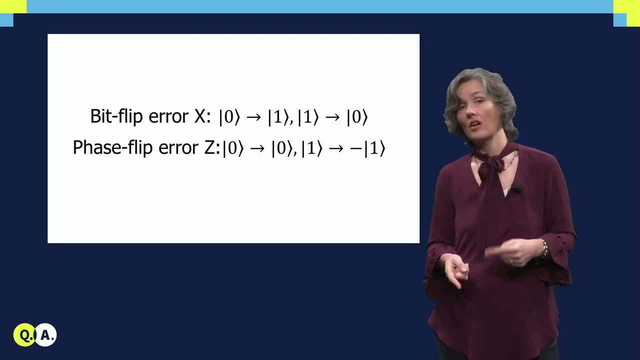 But wait, we can't just correct any old error. First of all, a qubit can undergo two types of elementary error. There is bit flip and there are phase flip errors. All other errors on a single qubit are linear combinations and or products of these errors. 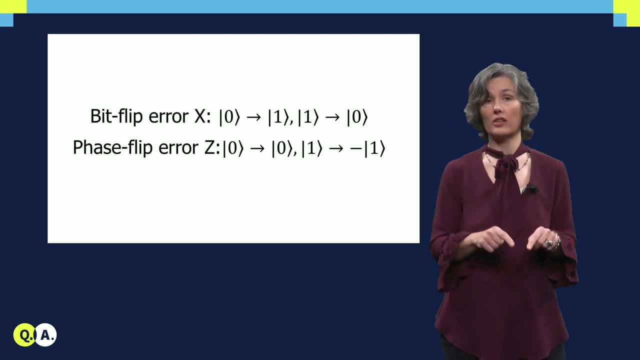 Quantum error correction codes are designed such that only errors on small subsets of qubits can be corrected. For example, for the seven qubits shown previously, an error on any single qubit can be corrected, but not an error on any subset of two or more qubits.